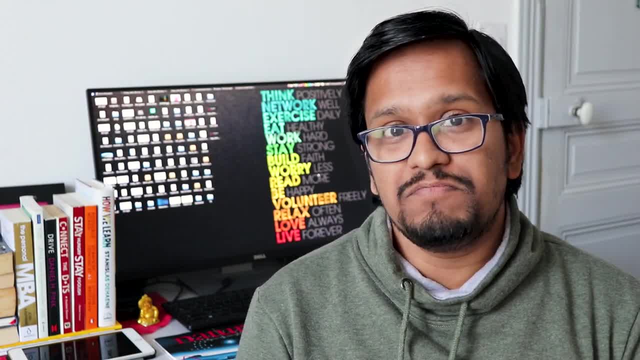 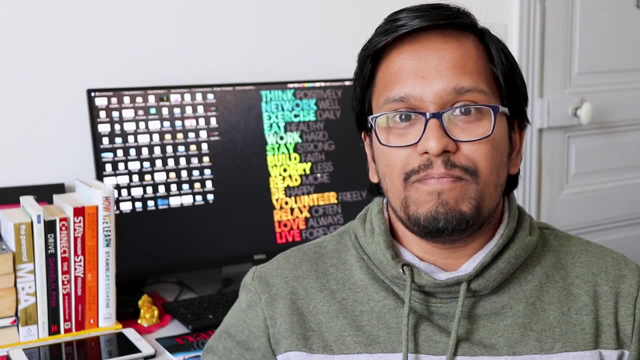 learning agent can be used to train a dog or a dog trainer. to train a dog trainer. to train a dog, The dog tries to figure out the quality of its action based on the rewards it receives, so that it can decide which actions to perform in sequence to get maximum reward in the long term. Let's 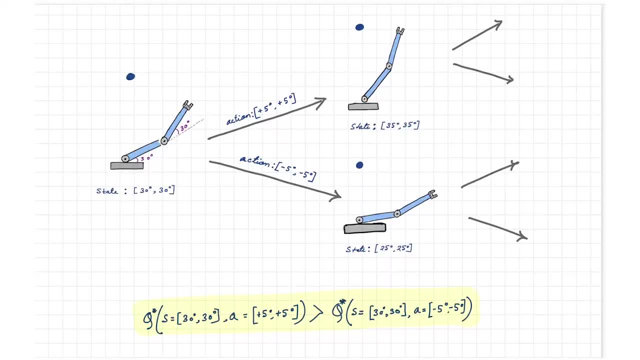 develop a quick intuition about Q-learning. Suppose this arm has to train itself to reach the target location with minimum number of steps. Let's assume that the arm receives a reward based on its distance from the goal. The smaller the distance, the higher the reward. The state of the 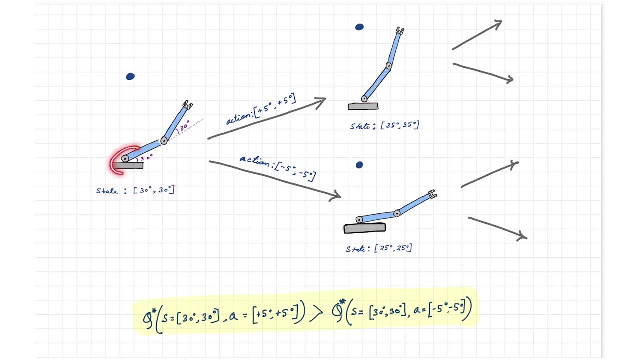 arm can be defined as its joint angles, since we are using a kinematic arm, so we are not considering any inertia, So our state can be defined fully using the joint angles. For instance, the current state of the arm can be written as a tuple of two values like 30 degrees and 30 degrees. Now, 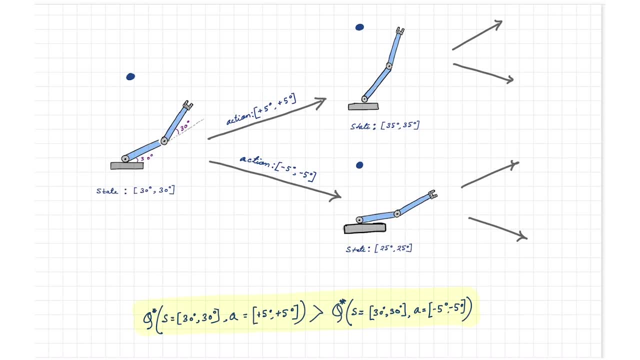 at this state. let's assume that the arm has two options: It can apply action positive- 5 degrees or negative 5 degrees. Let's assume that the arm has two options: It can apply action positive 5 degrees or negative 5 degrees. 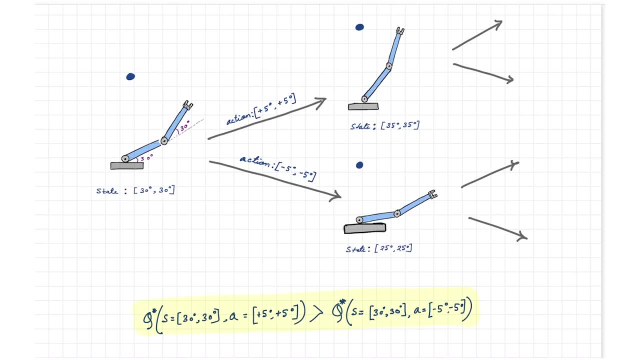 displacement to both the joints. Now you tell me which action is better for the arm to achieve the goal. It is positive 5 action or negative 5 action to the both joints. Exactly, it is the positive 5 actions to the both joints Because it will take the arm a bit closer to the target and give 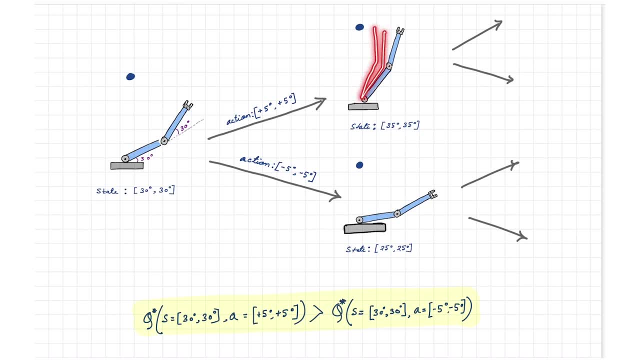 higher rewards in the long term if it decides the future actions also rationally. In terms of Q-values, we can say that positive five action has higher value compared to negative five action actions at the current state of 30 degree, 30 degrees of the arm. 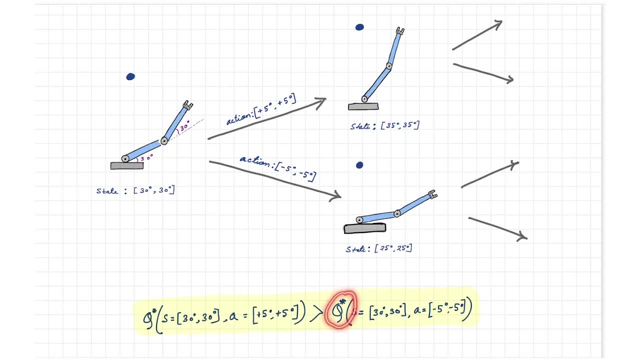 Q-learning attempts to figure out or estimate these values for all the possible actions, for all the possible states, so that the robot can decide optimally which action is the best to take at any state, depending upon the goal. Once the Q values are estimated, the arm can simply follow the action at any state that has highest Q value. 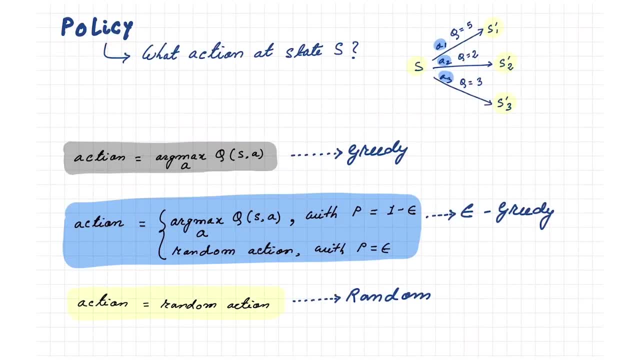 Now, in this case, the rule that decides a particular action based on the Q values is called the policy. For instance, a greedy policy always selects the action having the highest Q value at any state. Similarly, an epsilon greedy policy will select most of the time the highest Q value action. 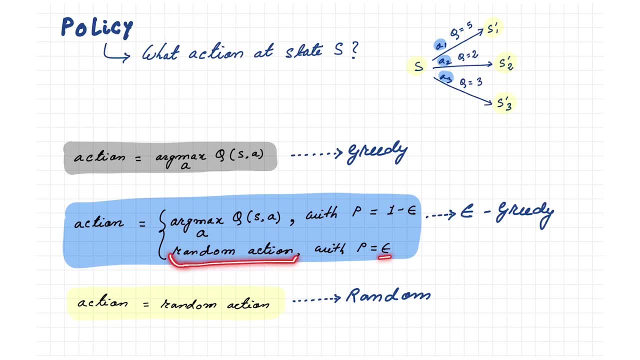 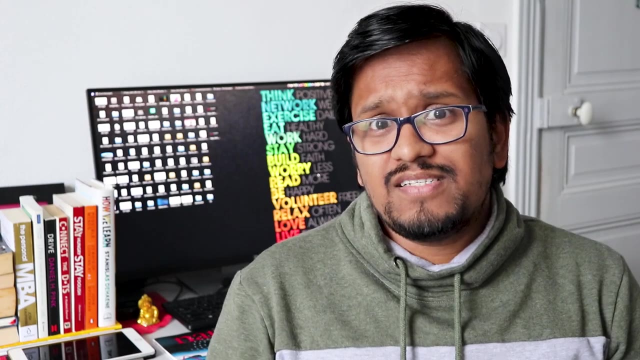 but sometimes selects any action randomly with a small probability epsilon. On the other hand, a fully random policy doesn't care about the Q values. It selects any action randomly at any state. I think basics are done now, So let's dive deeper into the game. 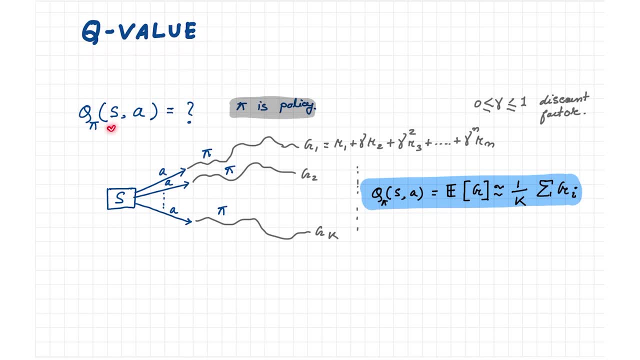 The formal definition of a Q value at any state S and for any action A corresponding to any policy. pi is the expected return received by the agent if it applies action A first and then it follows the policy. So it's a complicated policy, It's a complicated statement. 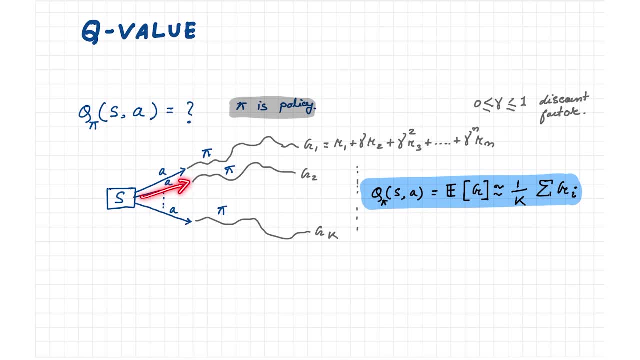 So the agent has to apply an action A first in state S and then onwards it has to follow the policy pi Okay, And doing so repeatedly. whatever rewards it gets, longterm rewards it gets, uh, the expectation of that- is called the Q value of the state and action pair. 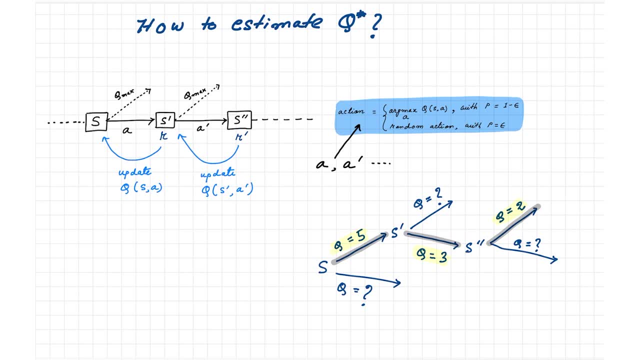 Now the question is how a robot or an agent autonomously figure out these optimal Q values. Here comes the Q learning update rule. The agent or the robot executes actions on the states it encounters using a behavior policy and after it sees the consequence of an action. 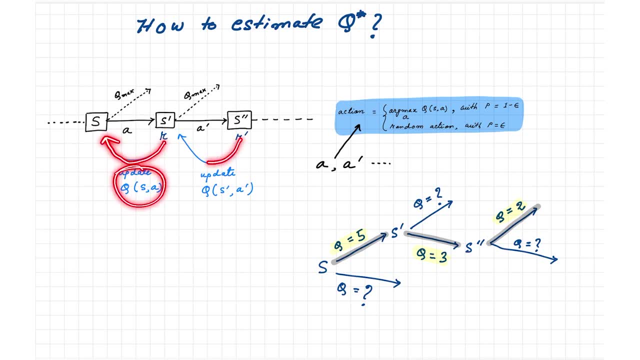 it updates the Q value of the action for the previous state. A behavior policy is any policy that allows the agent to explore wide range of actions for a wide range of states. For instance, we can use an epsilon greedy policy like this, As you can see, for any state, as this policy will tell the agent to perform mostly. 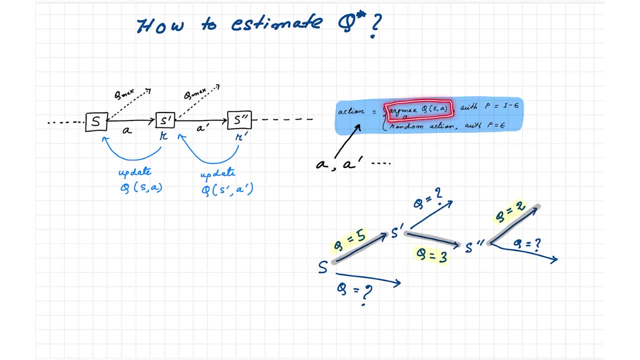 the action having maximum Q value, as I explained before, but sometimes with a small probability, epsilon, it will tell the agent to perform any random action. because of these random actions, the agent will not execute the same action sequence again and again because it has to explore all the states. 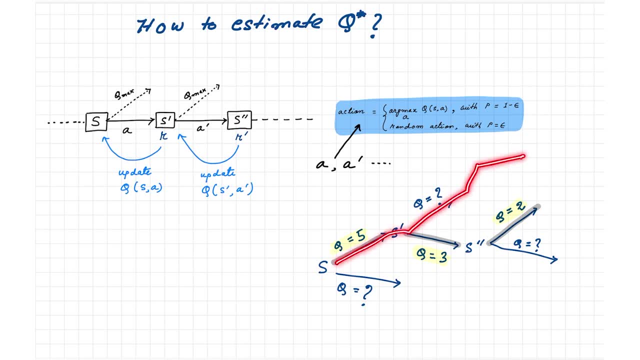 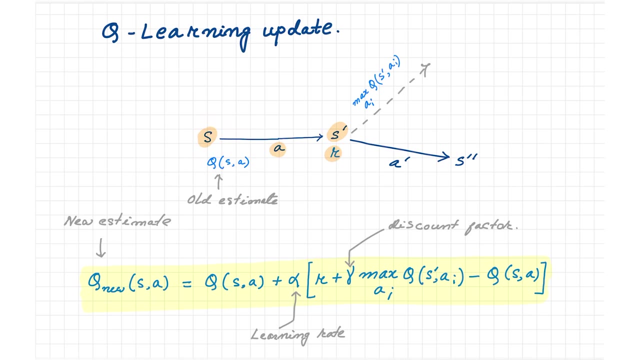 all the actions as widely as possible to estimate the Q values for all the possible state action pairs. Right now I guess we have enough knowledge about the background to talk about the update rule. Suppose, at any state as the agent executes an action, a as a consequence. 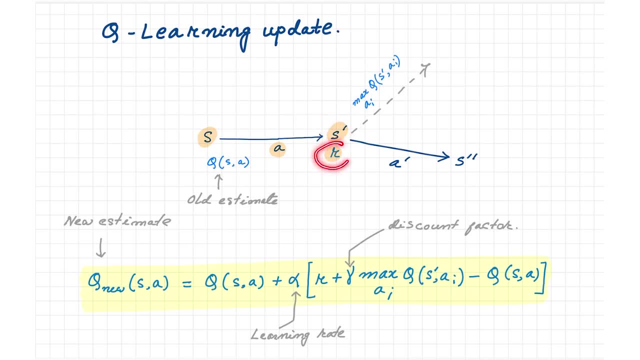 it moves to the state as dash and receive a reward, are then Q learning updates the Q value of the previous state like this: In this expression this is called the target Q value for the previous state. As you can see, the old Q value of the previous state is updated towards a fully greedy policy. 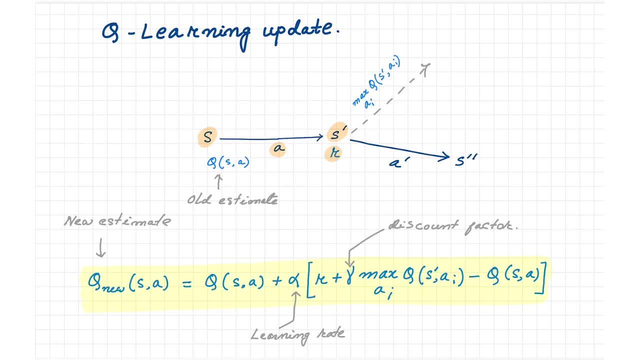 right Because, unlike Sarsa algorithm that we explained in the previous video, here we consider the Q value that is maximum in the next state, while in Sarsa we consider the Q value for the action that we actually take in the next state. 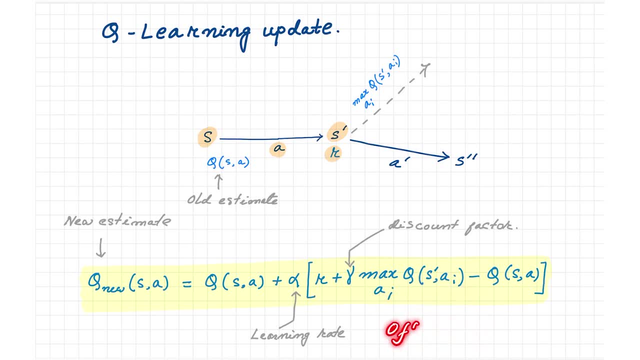 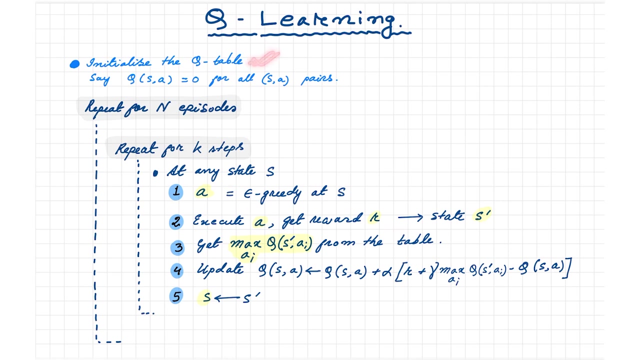 So Q learning is called off policy algorithm. We update the Q values towards the greedy target policy and not towards the policy that we are actually following. Here is the full Q learning algorithm. First we initialize the Q table with some arbitrary values for all the state. 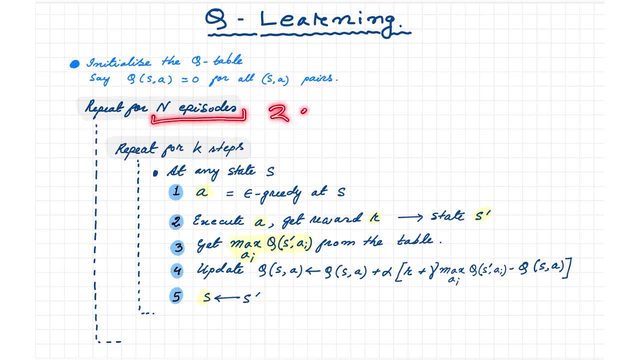 action pairs. Then we iterate for an episodes. At each episode we start from the initial state and we perform the action as an example. We start from K steps. if we do not encounter the terminal state at any state as first, we query the epsilon greedy policy a. 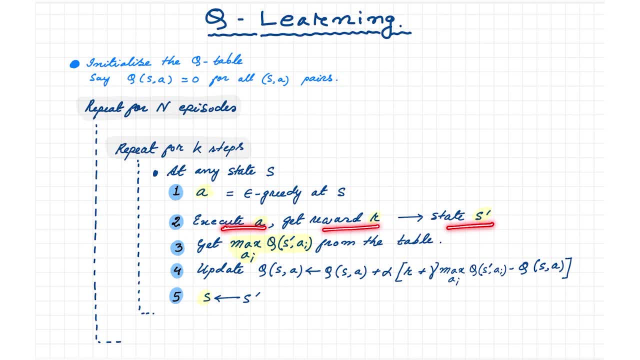 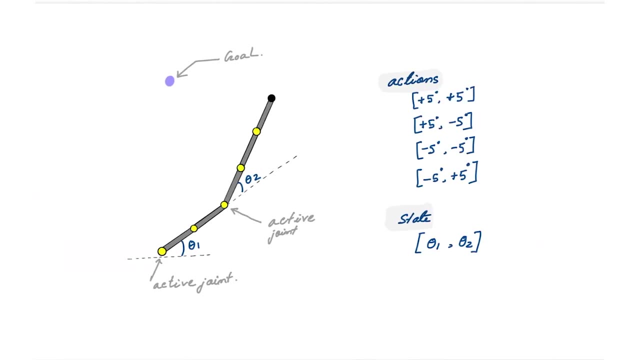 then we apply the action and observe the reward and the next state as dash. Then we update the old Q value for the previous state in the Q table using the Q learning update rule. Now let's apply the Q learning algorithm on a two degree of freedom: kinematic. 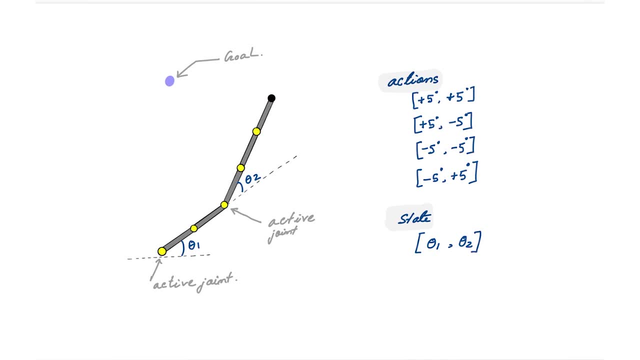 arm and see how it learns. The state of the arm can be defined, as I explained before, by a vector of its joint angles. The action is a vector containing positive or negative five degree displacement of the joints and the goal of the arm is to learn to reach this target. as 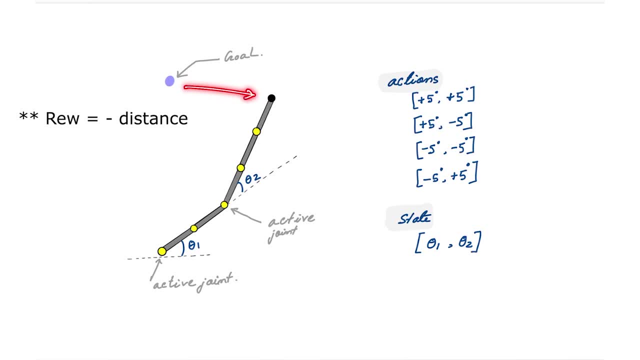 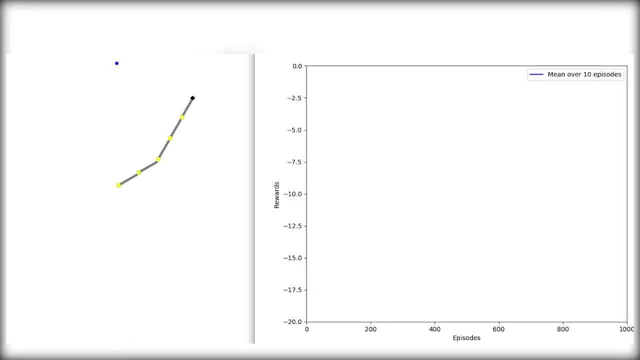 quickly as possible. So we give reward which is like inversely proportional to the distance, like we discussed before. Since Q learning requires discrete states, we discretize the states of the arm by an interval of 10 degrees. As you can see, the arm has started exploring with an epsilon greedy policy. 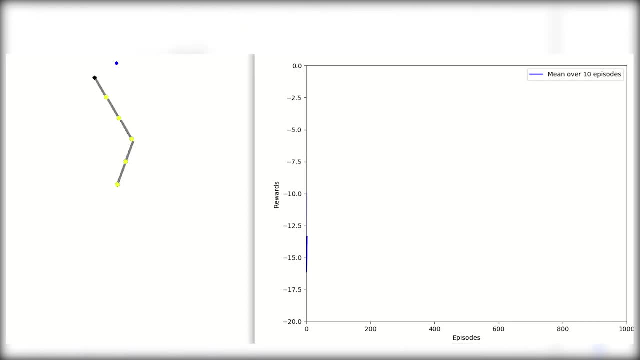 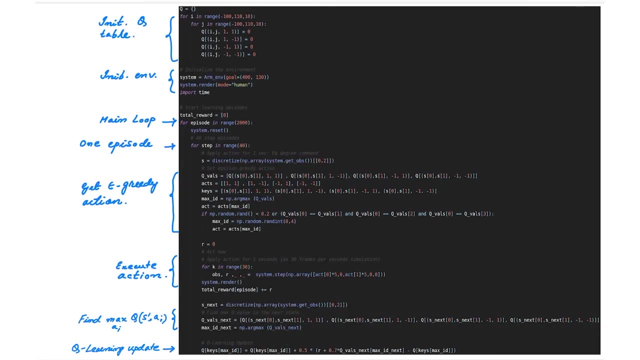 Since, initially, we do not have a good estimate of the Q values, the arm is moving mostly here and there without any significant reward collection While it is learning. let's have a quick look at the Python code that I have written for this. I made it as short as possible and didn't use any additional functions in the